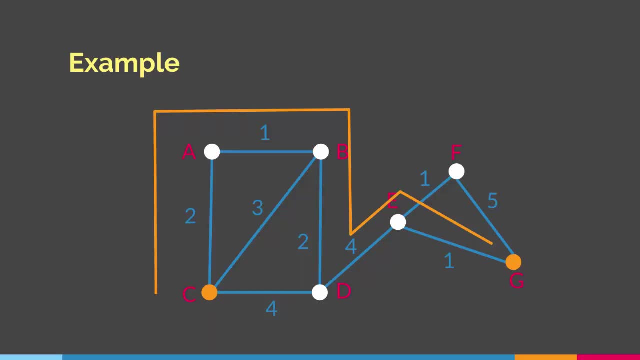 Or I can go like this: I can go from C to A to B to D to E to G. As you can see, in this particular path, the total sum of the weights of the edges in the path will be 2 plus 1, 3, 3 plus 2, 5, 5 plus 4, 9, 9 plus 1 is 10.. 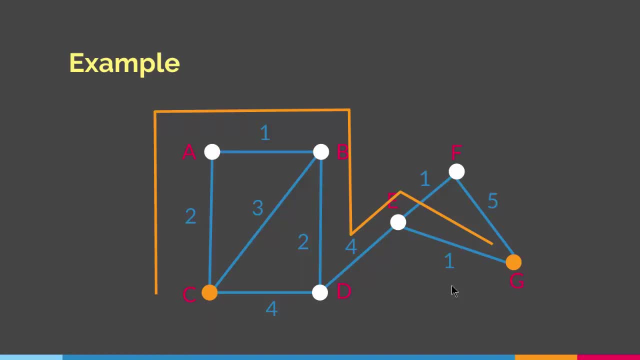 So, between all the paths that I have taken to go from C to G, this path is the shortest because the sum of the edges will be 9.. And the rest of the paths will be 10.. The rest of the paths that I took have the total sum of 10.. 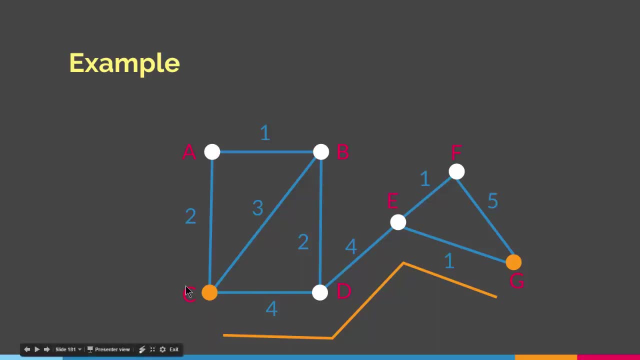 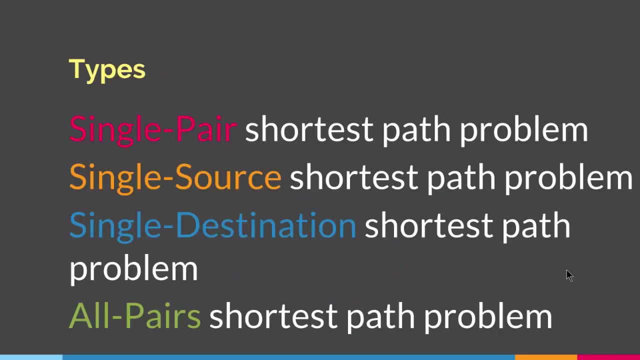 Therefore, the shortest path between C to G is a path that goes from C to D to E to G, And that is basically the idea of the shortest path problem. We have several types of shortest path problems. We have single pair shortest path problem. 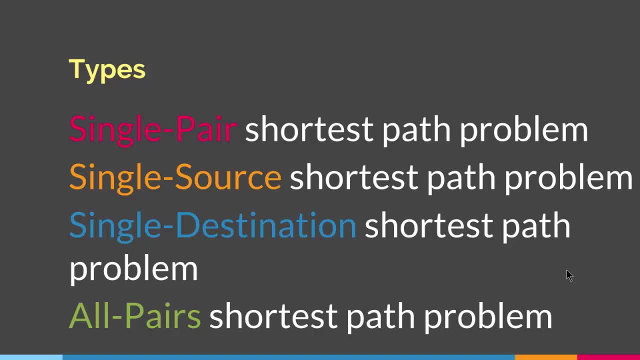 We have single source shortest path problem. We have single destination shortest path problem And we have all pairs shortest path problem. The single pair shortest path problem is finding a path. The shortest path problem is finding the shortest path between a single pair of vertices. 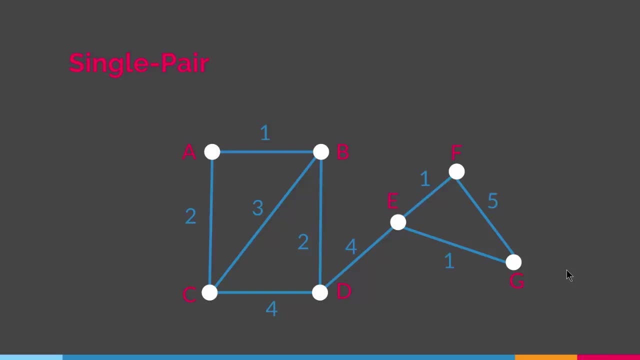 So let's say this is our graph: A single pair shortest path. problem will be finding the shortest path between C and F or between A and G. Basically, you take a single pair of vertices or points and you will find the shortest path between them. 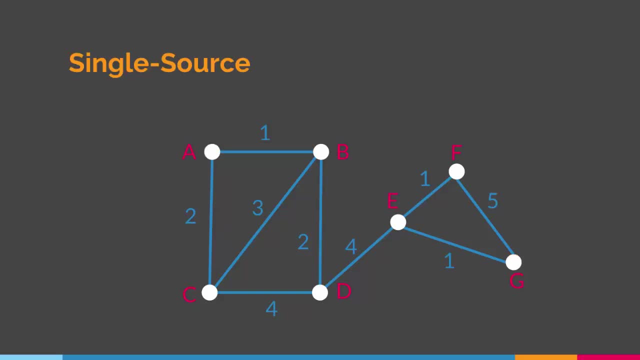 However single source, shortest path problem is pinpointing a vertex to be your source and then finding the shortest path from your source to all the other vertices. So here our source is C. I will find the shortest path between C and A, C and B, C and D, C and E, C and F and C and G. 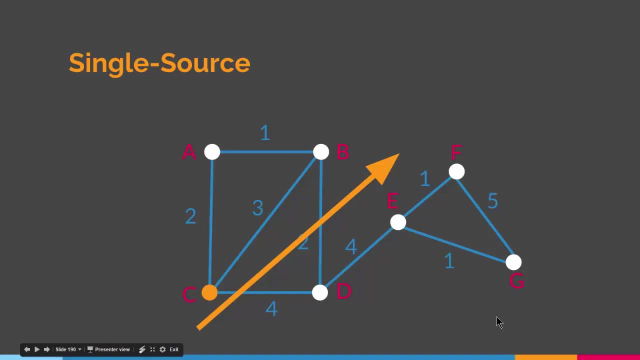 So the paths in the single source shortest path problem will originate from the source and it will head to the rest of the vertices. Then we have single destination- shortest path problem, which is opposite to the single source shortest path problem, And basically here you will have a destination. 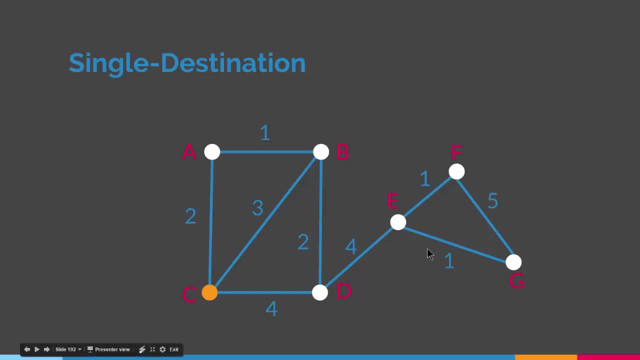 For example, let's say C And then you will find the shortest path from all the vertices, All the other vertices to C. In single source- shortest path problem: we found the shortest path from the source to the rest of the vertices. However, in single destination shortest path problem: we find the shortest path from the rest of the vertices to our destination. 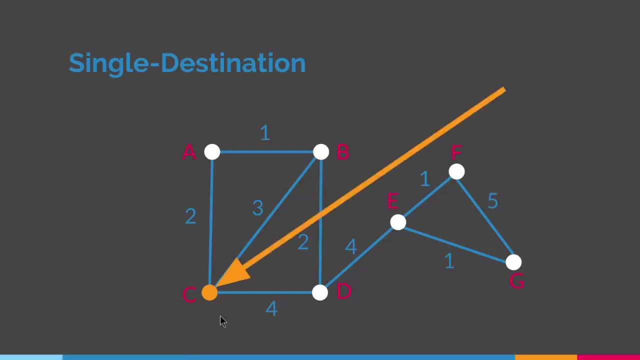 Here our destination is C, So the paths in single destination shortest path problem will originate from the other vertices to your destination. In our case it's C. Finally, we have all the vertices demiş. Next we will discuss the single pair shortest path problem, which is finding the shortest path between all the vertices. 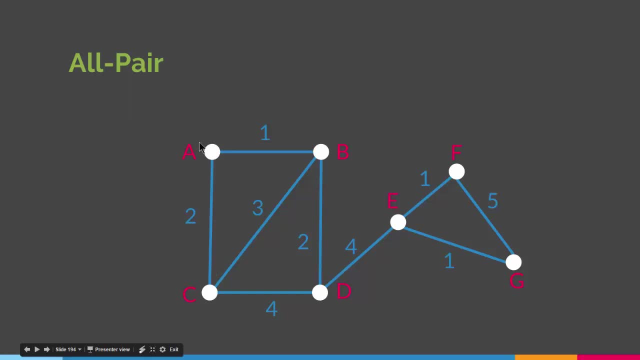 So let's say I will find the shortest path between C and D, C, D, D, F and G, then I will find the shortest path from B to C, C, A to D, E to D, F, A and G, then I will find the shortest path from D to C, C to D, A to D, E to D, F to D, E to F, and so forth, until I find the shortest path between all my vertices. 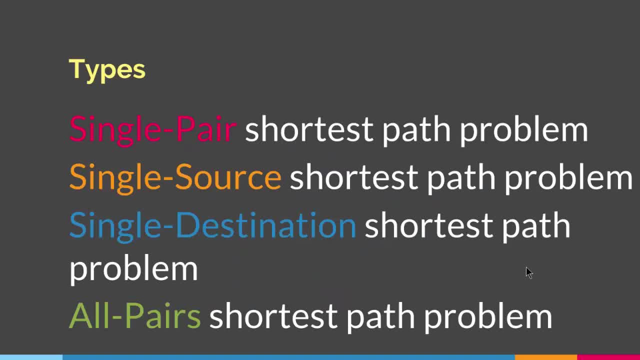 We have a set of single pair short path problems: path problem, which is finding the shortest path between a single pair of vertices. we have single source shortest path problem, which is dedicating a vertex to be your source and then you will find the shortest path from your source to all the other vertices. we have single destination shortest. 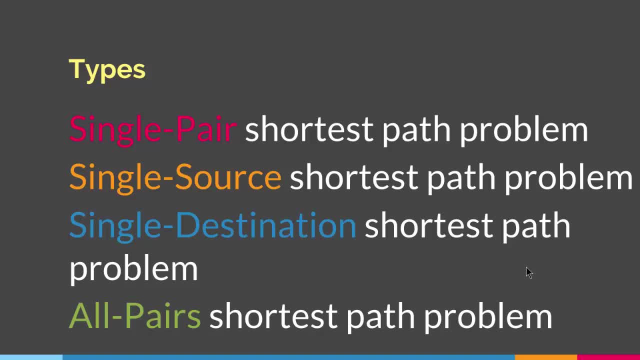 path problem, which is finding the shortest path from all the vertices to one single destination. and finally, we have all pairs shortest path problem, which is finding the shortest path between all your vertices. So now we know the types of shortest path problems. what are some of the ways? 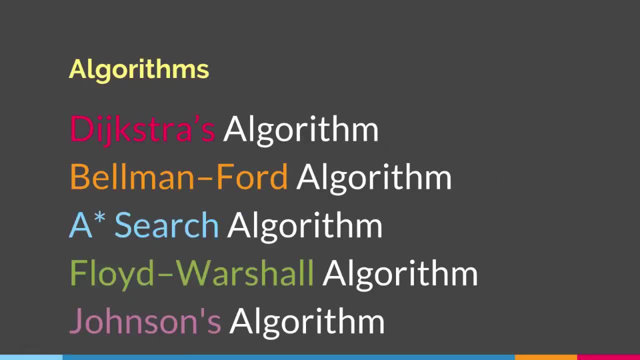 or algorithms that we can find a shortest path in a graph. Well, we have a couple of algorithms: We have Dijkstra's algorithm, we have Bellman-Ford algorithm, we have A-star search algorithm, we have Floyd-Warshall algorithm and we have Johnson's algorithm, such that all of these are used in order. 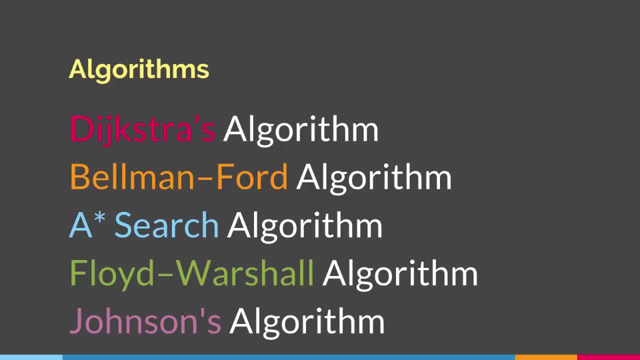 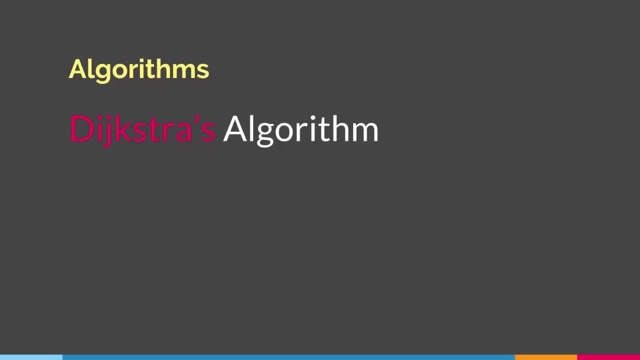 to find the shortest path in a graph. We will talk about Dijkstra's algorithm and we'll see how it is used in order to find the shortest path in a graph. So let me give an example on Dijkstra's algorithm. Let's say we have a graph like this: as you can see it, we have two, four, six vertices. 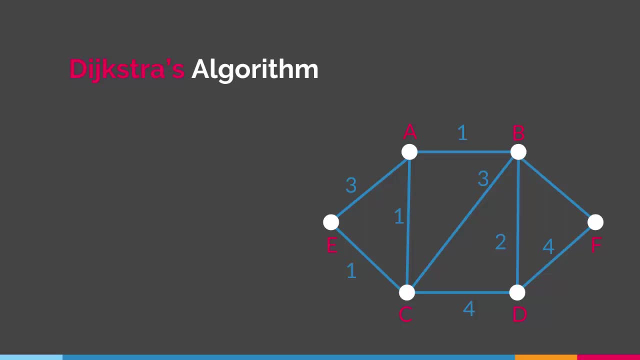 I have assigned a value to each edge and I'm trying to find the shortest path between E and F using Dijkstra's algorithm. So how does Dijkstra's algorithm work? Well, what I do in order to find the shortest path using Dijkstra's algorithm is: I'll assign values to each vertex. I'll assign 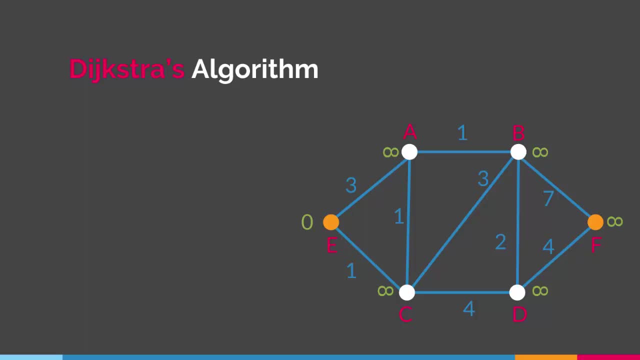 values to each vertex and I'll assign values to each vertex. So I'll assign values to each vertex, 0 to my initial vertex, and I will give infinity to the rest of the vertices. So here E has the value of 0, and A, C, D, B and F- all of them have value of infinity. Initially, that's what I do. 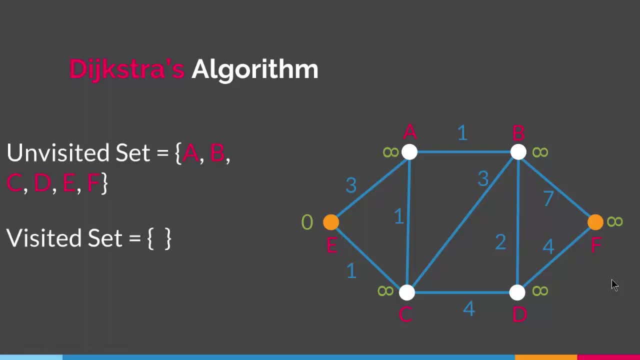 Then what I do is I'll create two sets. one of them is called unvisited set, and at the beginning it contains all my vertices. and one of them is called visited set, and initially it does not contain any vertices. As I move along, I'll create another set and I'll create another set, and at the beginning 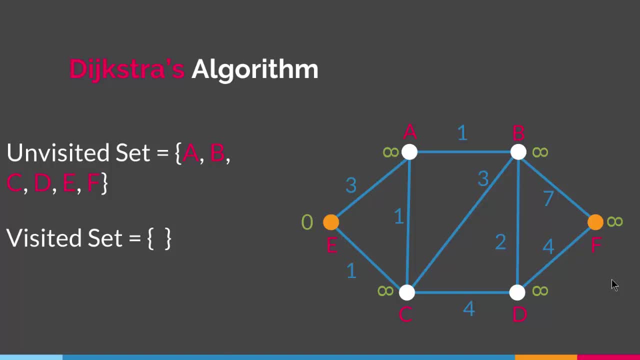 in finding the shortest path between E and F and visit. the set will decrease one by one and visit the set will increase one by one until I reach the end where the and visit the set does not contain anything and the visitor set contains all my vertices. after I do this, what I do is I will look at the vertices. 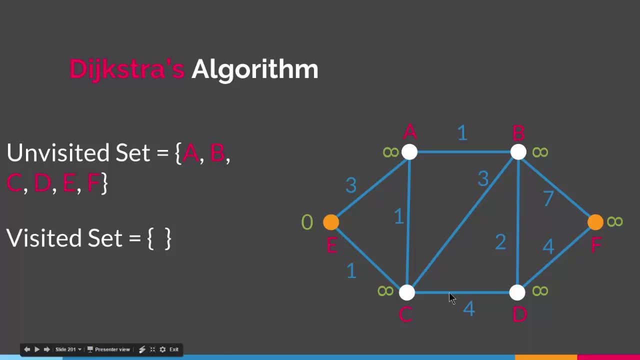 that are connected to my initial vertex. in this case, the vertices are connected to vertex e, our C and a. what I do is I will look at the value of A and C and C if their value is greater than the value of the edges that connect a and C to. 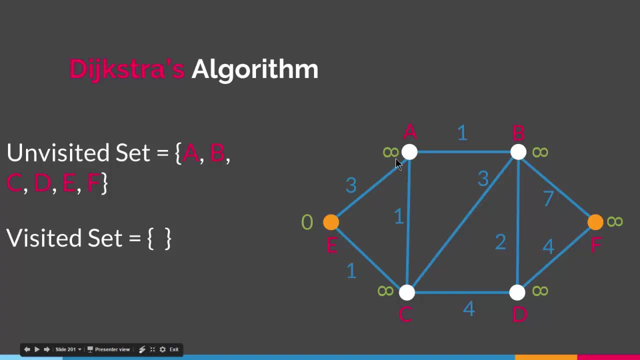 chewed. so in this case, the value of a is infinity. the value of the edge that connects a to e is 3. infinity is greater than 3 and in this case, infinity is greater than 1 when I have the value of a vertex greater than the edge or the. 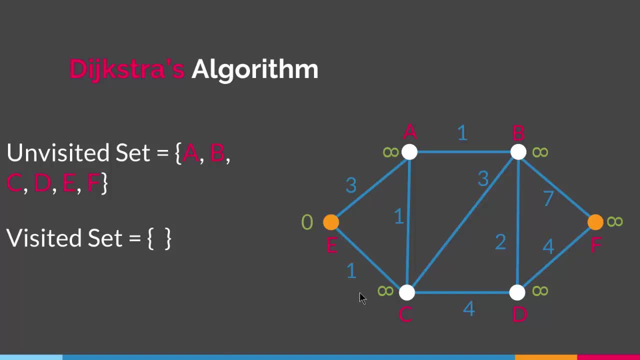 setting recognized. so, for example, I am connecting the edge at E to my initial. of the edges that they connect my initial vertex to that particular vertex, i will change the value of that particular vertex to the sum of the edges that connects my initial vertex to that particular. 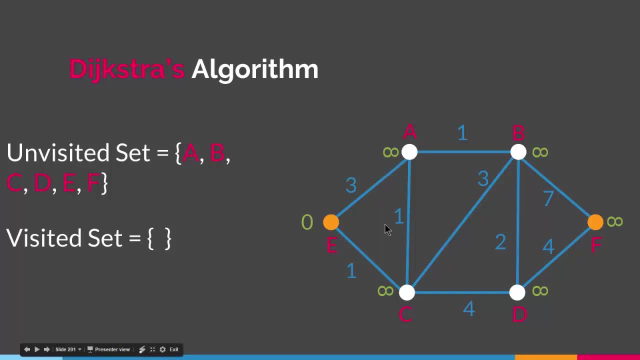 vertex. so here the value of a and c will change from infinity, to one of them having value of 3 and the other one having the value of 1.. after i decrease the value of the vertices that are connected to my initial vertex, i will mark my initial vertex as visited. so e comes from and. 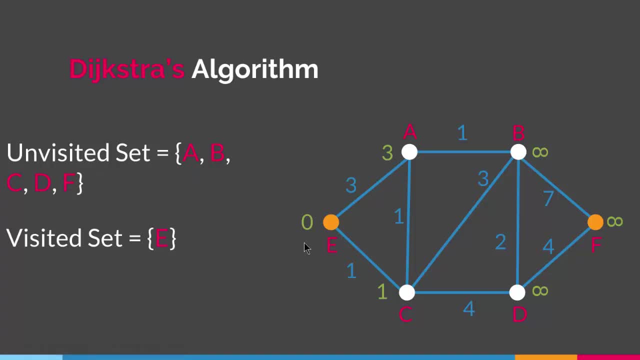 visit the set, to visit the set, and then i'll go to the vertex that has the smallest value- in this case i have to go to c- and then i will repeat the same step. we will look at the vertices that are connected to c- in this case they are a, b and d- and then we will change their values. 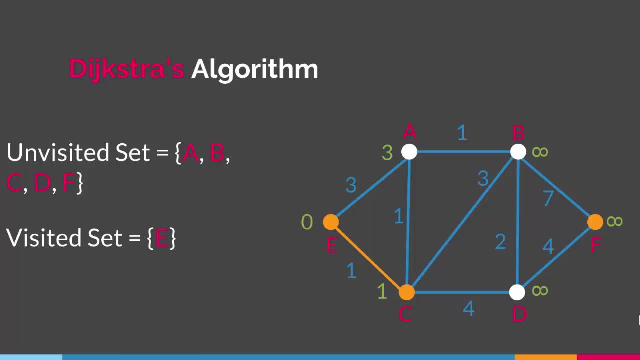 so we will change their values based on whether the current value that they have are great or just little bit greater than the sum of the edges that connect the initial vertex to that particular vertex. so here the initial vertex are e and e is connected to b through c, the value of 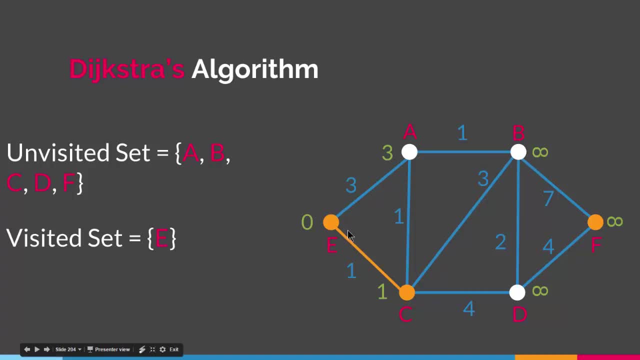 b is infinity and the sum of the edges that connect e to b through c are 1 plus 3, which is 4.. 4 is less than infinity. we will change the value of b from infinity to the value of the sum of the edges that connect e to b through c. 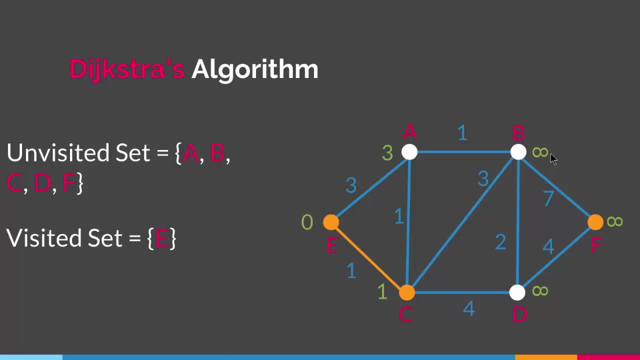 of b will be 4, the value of d will be 5 and the value of a will turn from 3 to 2. this is what happens. you may wonder why the value of a changed from 3 to 2. well, the initial value of a was. 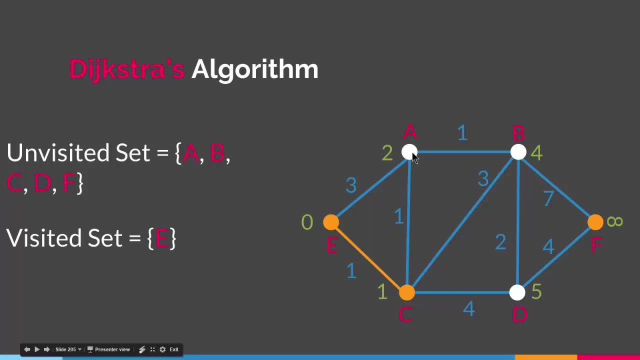 infinity. and then it became 3, since a is connected to c and there's a shorter path from e to a, which is through c. that will give the value of a to 2 instead of 3. so if you go directly from e to a, you will have the value of a to b3. however, if you go from e to c to a, you'll have the value of a to 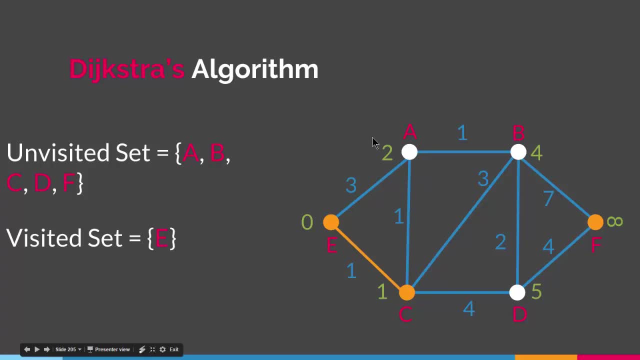 b2. since that is the case, we will change the value of a from 3 to 2, and the rule is: when the current value of a vertex is greater than the value of the sum of the edges that connects that particular vertex to the initial vertex through a vertex, then you will change the value of that particular. 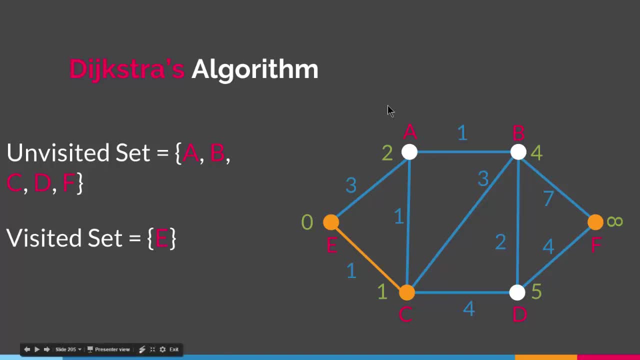 vertex to the new value. in this case, we change the value of a to 2 from 3, and then the value of b is 4 and the value of d is 5.. Once we determine the values of the vertices that are connected to c, we will mark vertex c as visited, and then we will go to the 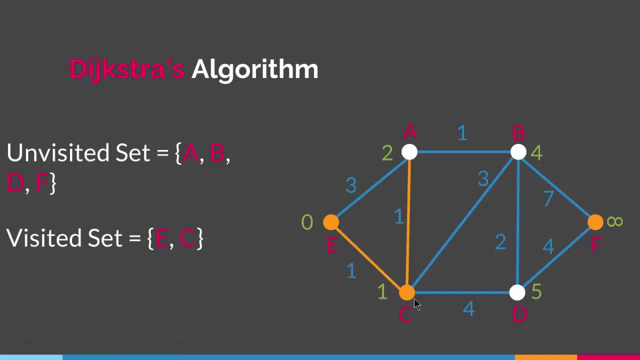 vertex that has the smallest value. In this case it is a. Okay, so now we will look at the vertices that are connected to a, and the only vertex that is connected to a that is unvisited is b, So we will go to b. However, if you notice, the value of b has to change because the sum of the edges that 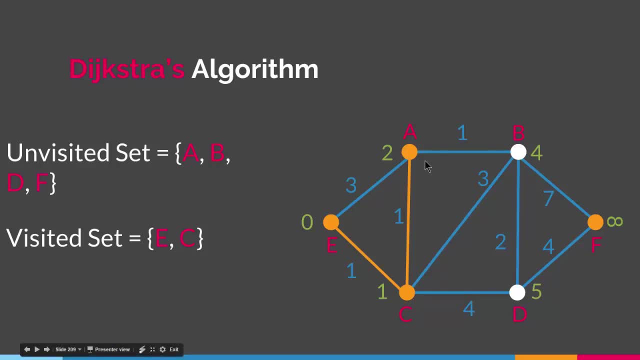 connects my initial vertex, which is e, to b, through the visited vertices, is 3, because 1 plus 1 plus 1 is 3.. 3 is less than the current value of b, which is 4.. Therefore, I have to change the value of b to 4, and that is what I exactly do, And then I'll go to b and, as you can see, I have 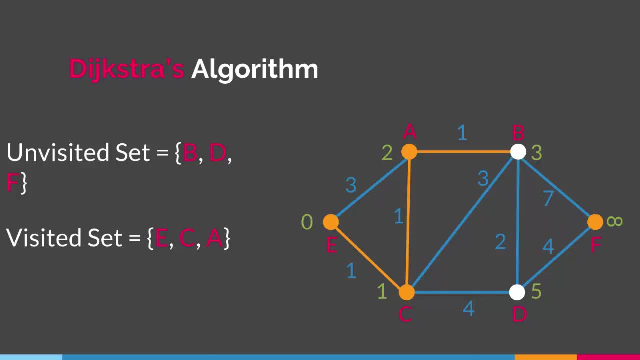 marked a as a visited set and then I'll look at the vertices that are connected to b. In this case they are c, d and f, and I'll try to change their values. However, since c is unvisited, I will go to b and, as you can see, I have marked a as a visited set, and then I'll 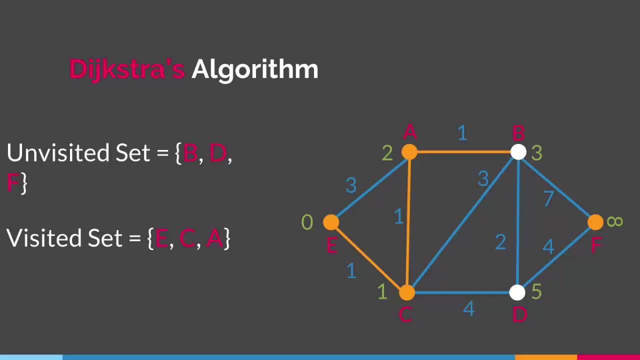 the visited set. I'm not going to try to change its value. I'm just going to try to change the value of d and f. The value of f definitely going to change. However, I don't know if I have to change the value of d, And changing the value of d depends on whether the value of the edges that. 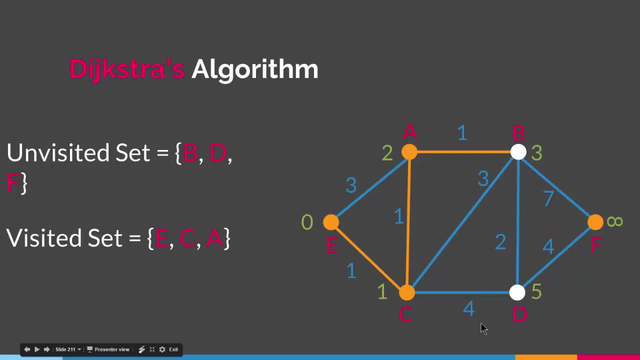 connects vertex d to e through the visited set is less than the value of d. If it is less than that, then I'll change the value of d to the new value. However, let's see if that is the case. Well, here we have 1 plus 1, 2 plus 1, 3.. 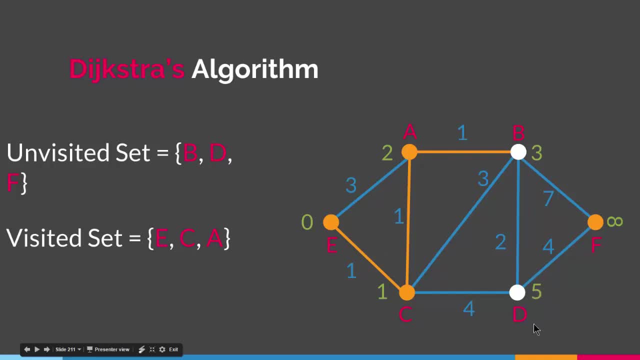 Plus 2 is 5.. Since 5 is equal to 5, I'm not going to change the value of d. However, I have to change the value of f from infinity to 10.. Since the sum of the edges that connects e to f through the 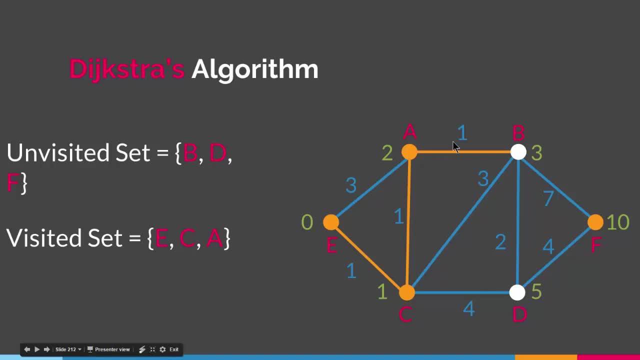 visited set is 10.. 1 plus 1 is 2 plus 1 is 3 plus 7 is 10.. Once I do that, I'll put b from the unvisited set to the visited set and then I'll go to the vertex that is connected to b and is not. 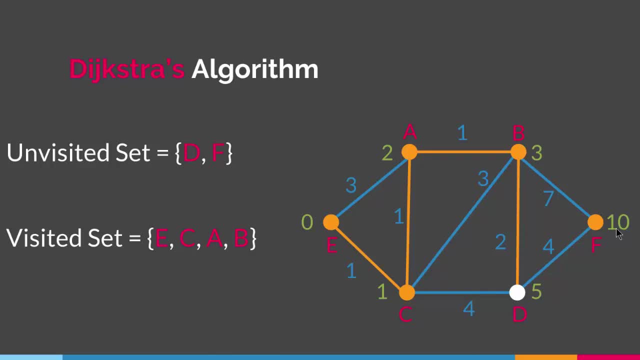 in the visited set and has the smallest value. In that case it is d. I'll go to d. and then I don't have an option, I have to go to f. in that case, Once I go to f, I'll mark f to be in the visited set. and now, since, as you can see it, I don't have any, 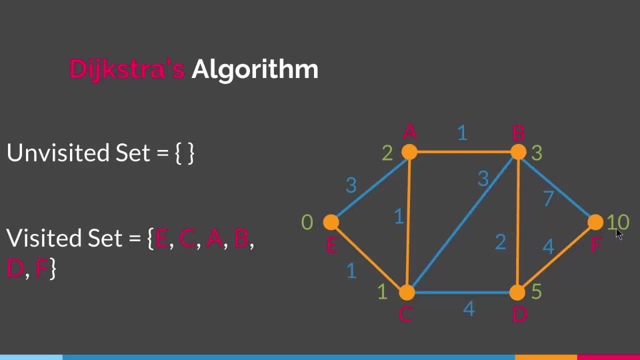 elements in the unvisited set and all my vertices are in the visited set. Now I have found the shortest path and I have to keep in mind to change the value of f from 10 to 9 because some of the edges that connects e to f from the visited set equals 9 instead of 10.. 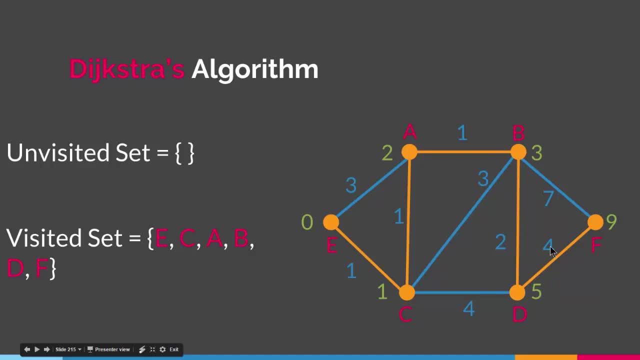 1 plus 1 is 2, plus 1 is 3, plus 2 is 5, plus 4 is 9.. If I go from b to f directly, I'll have the value of 10.. If I go from b to f through d, I'll have the value of 9.. And this is the shortest path from e.